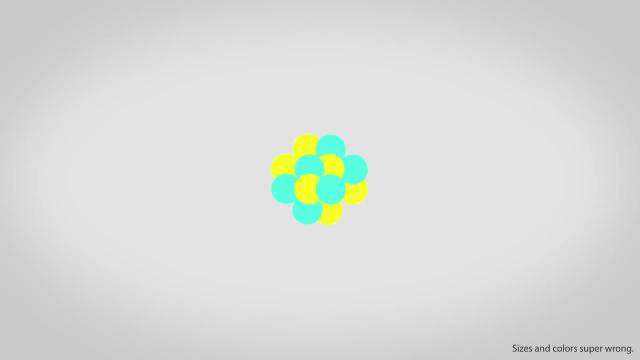 Protons and neutrons bind together and form the atom core, held together by the strong interaction, one of the four fundamental forces in the universe. They are made from quarks And held together by gluons. Nobody knows exactly how small quarks are. 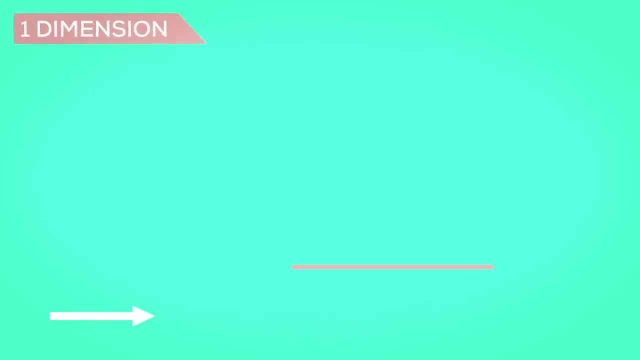 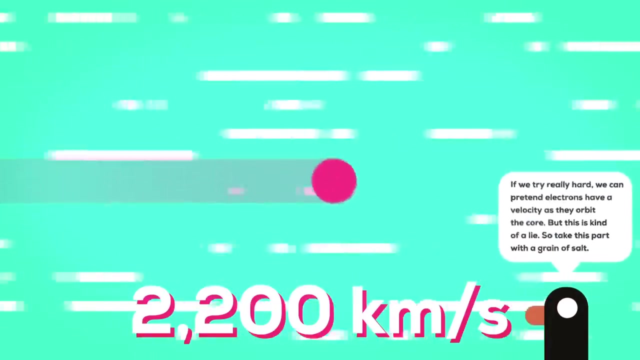 We think they might literally be points like in geometry. Try to imagine them as being zero-dimensional. We suspect that quarks and electrons are the most fundamental components of matter in the universe. Electrons orbit the atom core. They travel at a speed of about 2,200 kilometers per second. 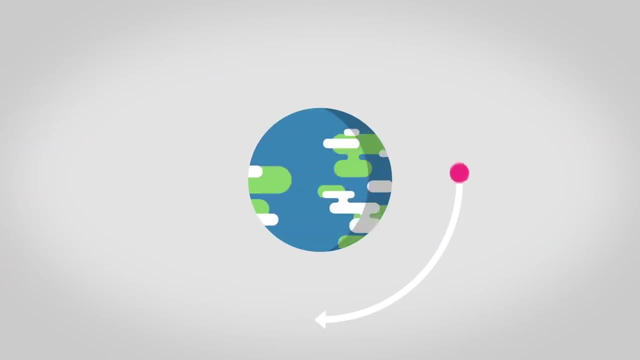 Fast enough to get around the Earth in just over 18 seconds. Like quarks, we think electrons are fun. Like quarks, we think electrons are fun. So they are the fundamental particles. 99.9999999999999999% of an atom's volume is just empty space. 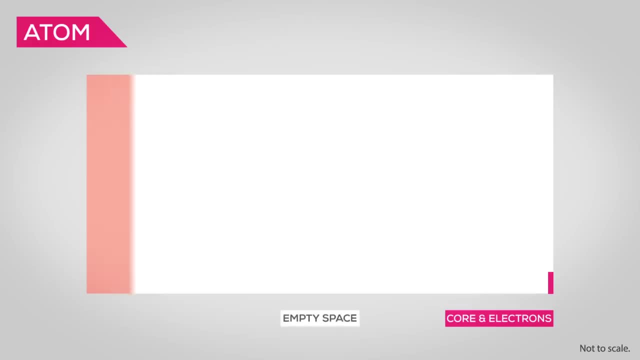 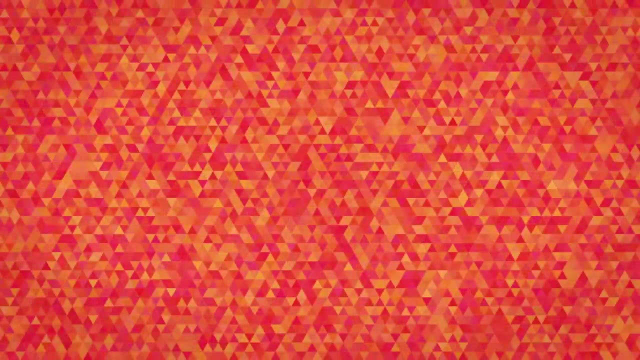 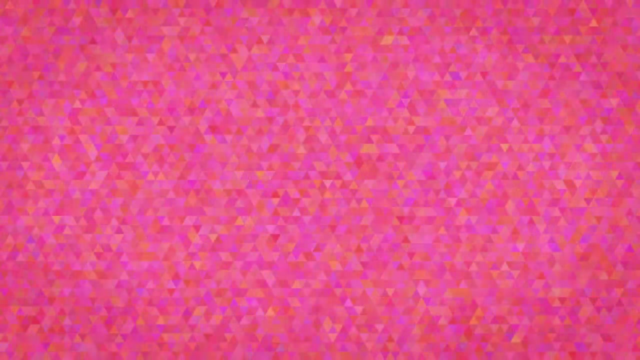 Except that it isn't. What we perceive as emptiness is actually a space filled by quantum fluctuations, fields that have potential energy and build and dissolve spontaneously. These fluctuations have a fundamental impact on how charged particles interact, but that's a topic for another video. 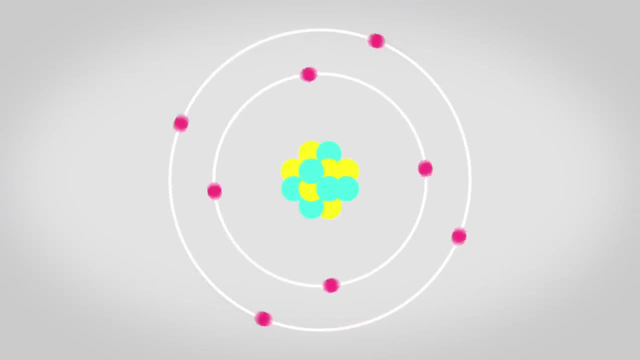 How much space do the core and electrons actually fill? If you were to subtract all the spaces between the atom cores from the Empire State Building, it would be about as big as a rice corn. All the atoms of humanity would fit in a teaspoon. 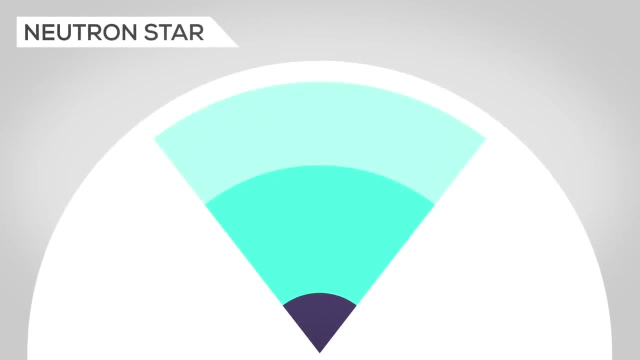 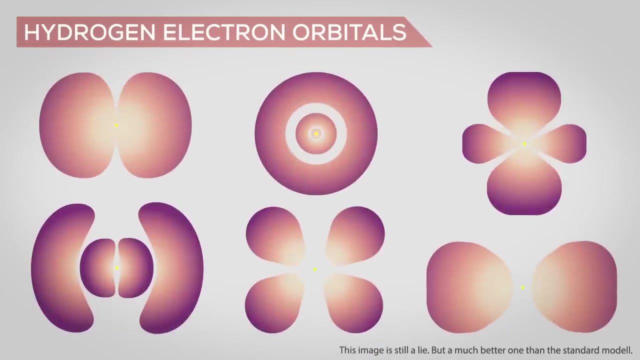 There are extreme objects where states like this actually exist. In a neutron star, atom cores are compacted so densely that the mass of three suns fits into an object only a few kilometers wide. By the way, what do atoms look like? Well, kind of like this. 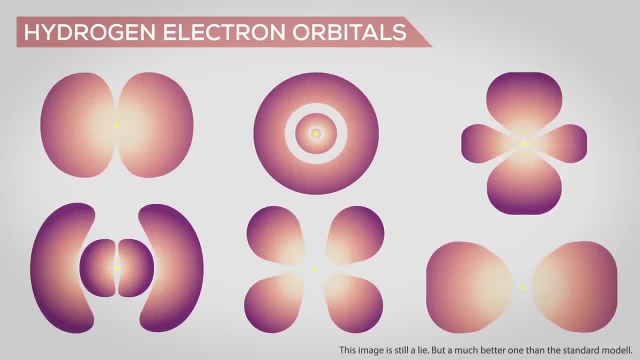 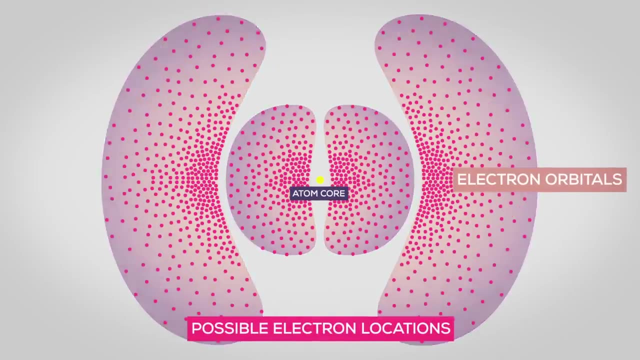 Electrons are like a wave function and a particle at the same time. We can calculate where an electron might be at any given moment in time. These clouds of probability, called orbitals, are where electrons might be with a certainty of 95%. 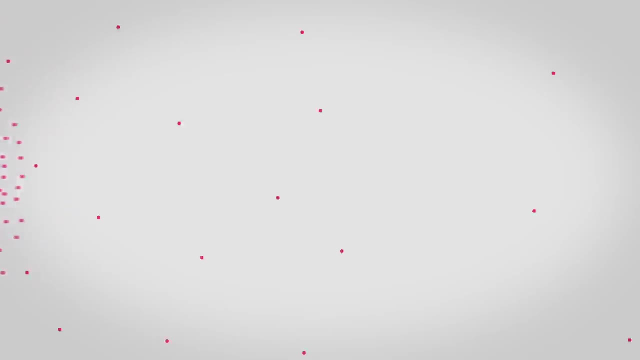 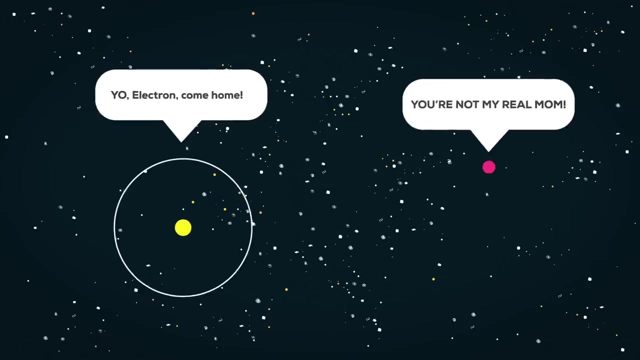 The probability of finding an electron approaches zero the further we get away from the atom core, But it actually never is zero, which means that, in theory, the electron of an atom could be on the other side of the universe. Okay, wait a second.